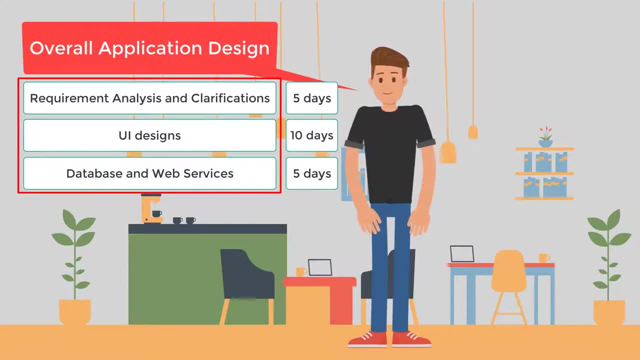 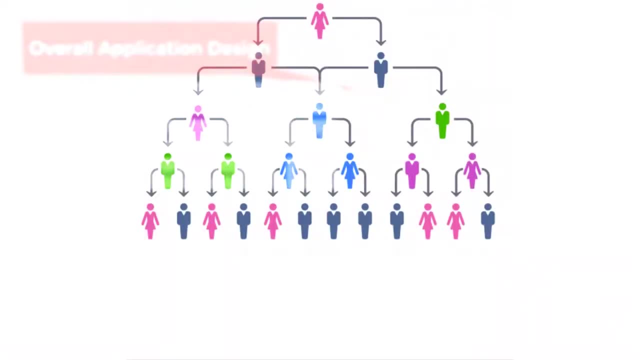 as throughout the life cycle of the project, Requirements analysis helps to keep the requirements in line with the need of the business. The hierarchy normally we have in software companies is: CEO, Vice President, Senior Project Manager, Senior Product Manager, Senior Software Architect. 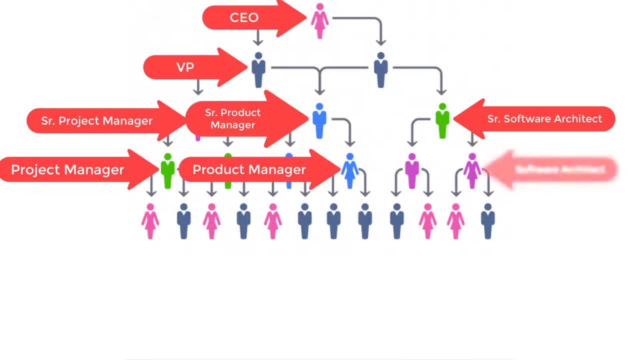 Project Manager, Product Manager, Software Architect. Now you have to complete the phase of overall application design. First, you have to complete the phase of overall application design: Requirement, analysis and clarification: 5 days. Database and web services: 5 days. Database and web services: 5 days For the success of a project you have. 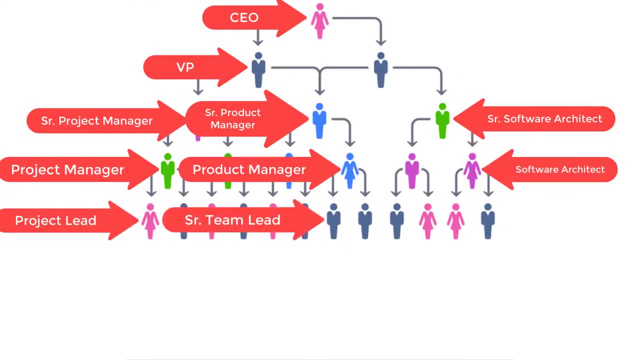 to complete the phase of overall application, design, Requirement analysis and clarification- 5 days. For the success of a project, you have to complete the phase of overall application, design, Requirement analysis and clarification- 5 days. Project Lead- Senior Team Lead. Senior Technical Lead- Module Lead- Team Lead- Technical Lead- Senior. 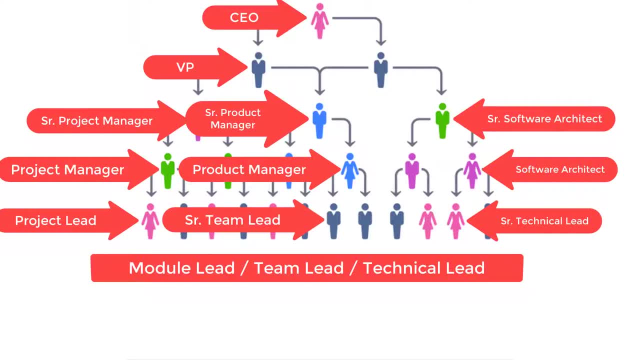 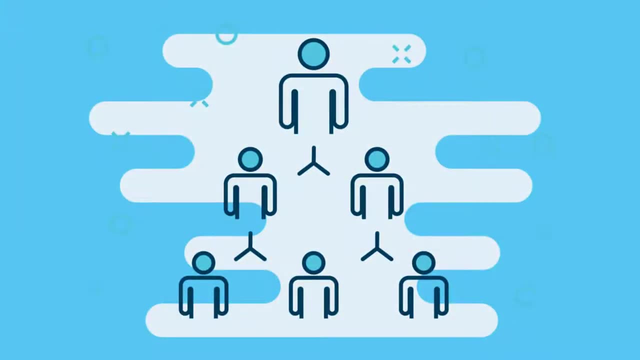 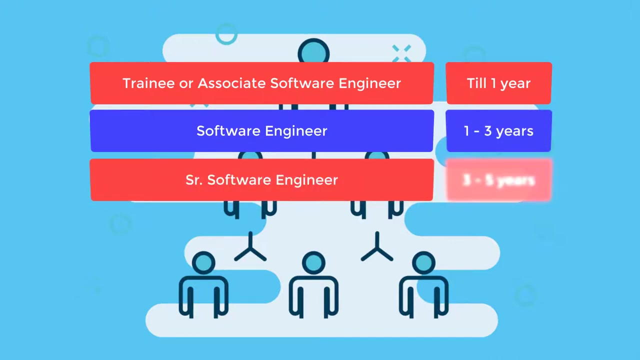 Software Engineer. Seniorkward Engineer Software Engineering. QA Engineer, System Engineering. Mary cleaner, Mar remarkable dürwy Normal these hierarchy have experienced, say, trainee or associate software engineer under one year. software engineer one, two, three years. senior software engineer. three to five years. technically lead engineer from three to five years or five. 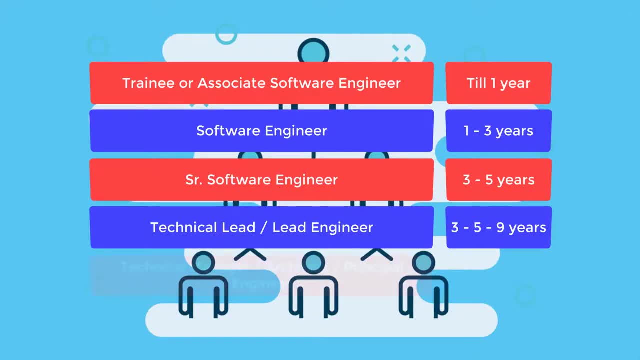 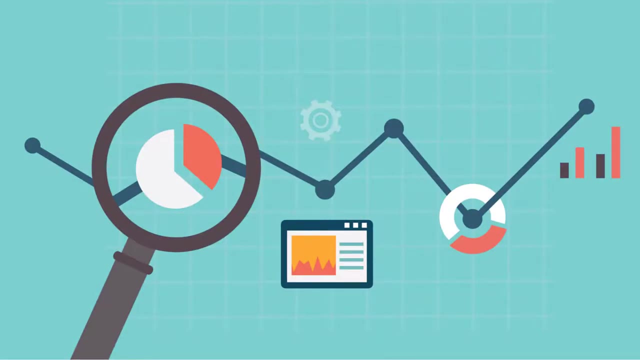 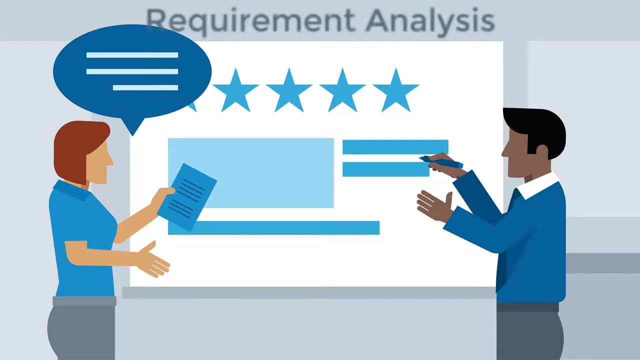 to nine years depend upon the company: technical manager, architect, principal engineer- at least nine years for the success of a project. it is at most important to analyze project requirements when they are gathered, as well as throughout the lifecycle of the project. requirements analysis helps to keep the requirements in line with the need of the business. a good requirements. 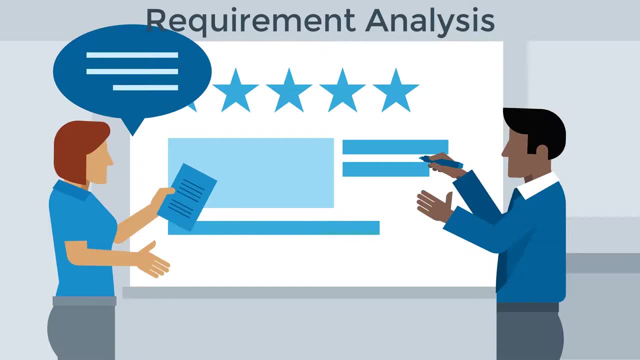 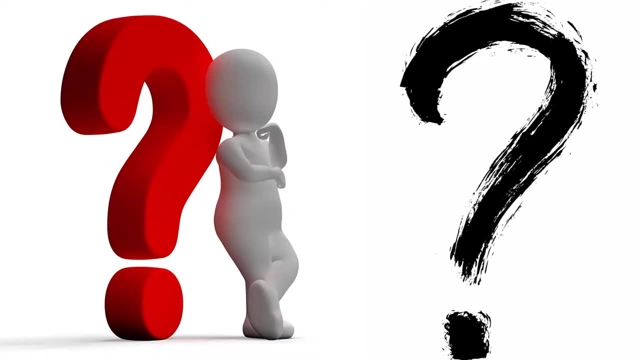 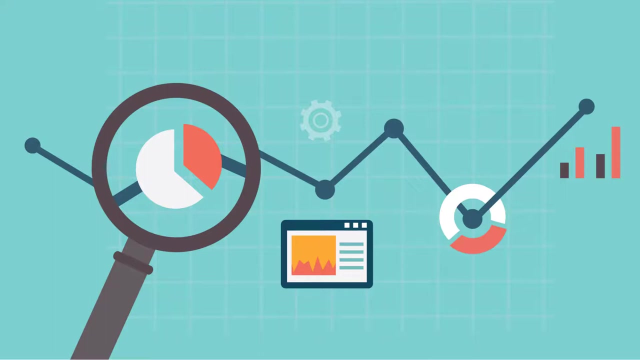 analysis process will render a software application that caters to the objectives of the business set for. have you read BRD? have you? you understand each and everything? are you clear about the requirements? share your analysis in comments. there are various techniques of requirement analysis. I tell a few of them: business process modeling, notation, unified modeling.